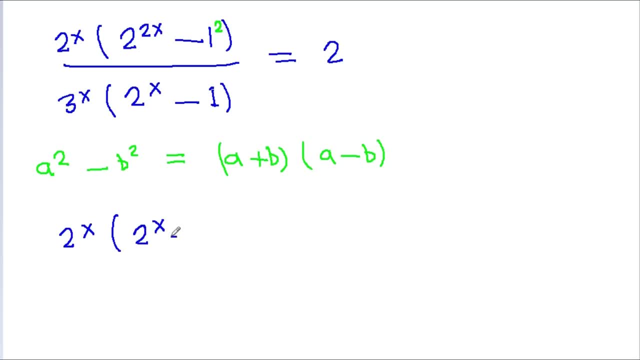 x minus 1 square will be 2 to the power x plus 1 into 2 to the power x minus 1 by 3 to the power x times 2 to the power x minus 1 is equal to 2.. And now we can cancel 2 to. 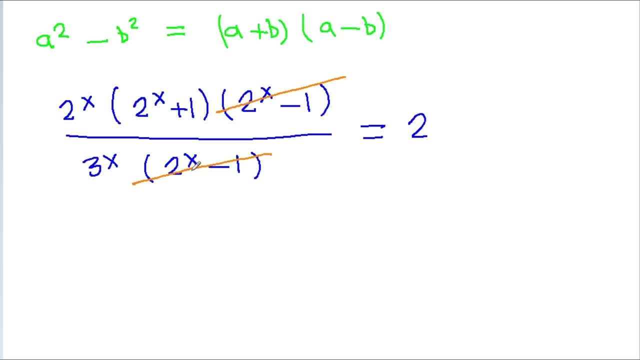 the power x minus 1 and 2 to the power x minus 1, provided if 2 to the power x minus 1 is not equal to 0. Or 2 to the power x not equal to 1 or x not equal to 0. And now we get 2 to the power. 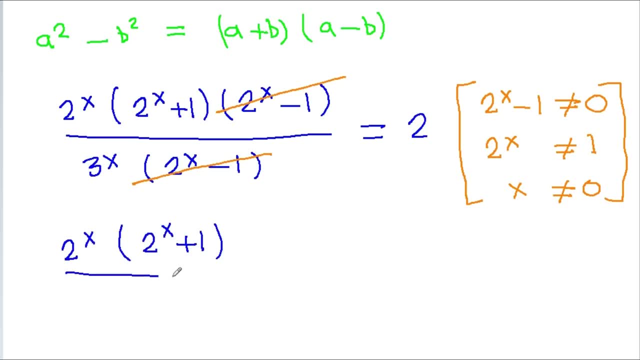 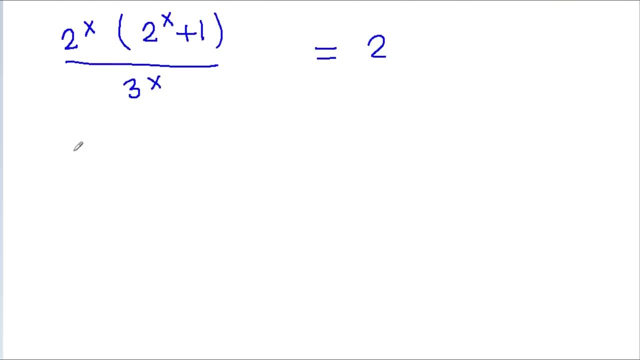 x into 2 to the power x minus 1 by 3 to the power x is equal to 2.. Or we get 2 to the power x times 2 to the power. x minus 1 is equal to 2.. And here, if we take 2 to the power, 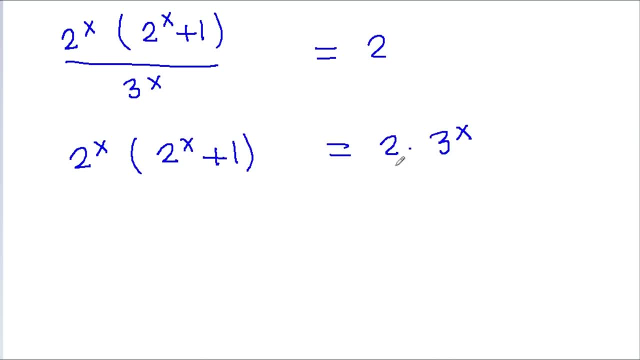 2 into 3 to the power x. and now if we divide by 2, then we get 2 to the power x minus 1 times 2 to the power x minus 1 is equal to 3 to the power x, and we know that x is not equal to 0. and now for x. 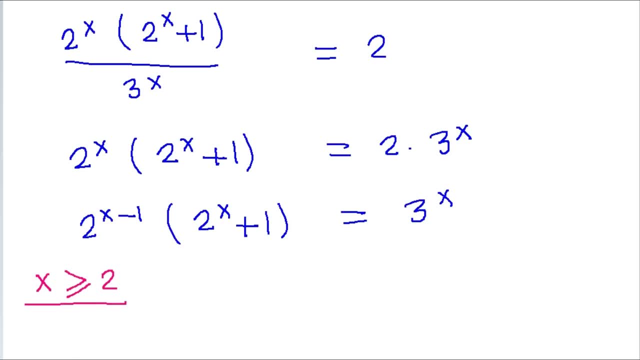 greater than or equal to 2. here we have 2 to the power x minus 1 into 2 to the power x minus 1 is equal to 3 to the power x and for x greater than equal to 2, 2 to the power x minus 1. 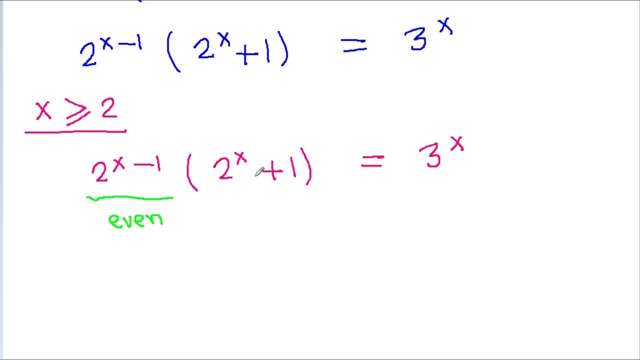 it will be even. and 2 to the power x minus 1, it will be odd, and even times odd is even. and 3 to the power x, it will be odd and even cannot be equal to odd. so no solution for x greater than equal to 2. and now: 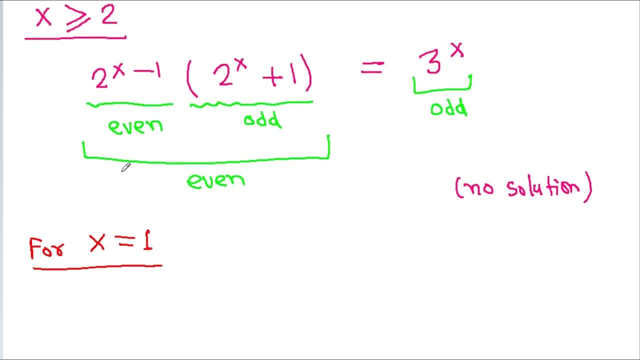 for x is equal to 1, we have 2 to the power x minus 1 times 2 to the power x minus 1 is equal to 3 to the power x minus 1 is equal to 3 to the power x and for x is equal to 1, it will be 2 to the power 1 minus 1. 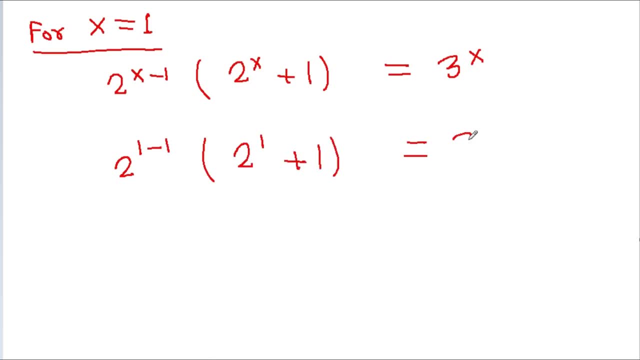 times 2 to the power 1 minus 1 is equal to 3 to the power 1 and 2 to the power. 1 minus 1 is 2 to the power 0. that will be 1 into 2 minus 1 will be 3 is equal to 3 and we get 3 is equal to 3. 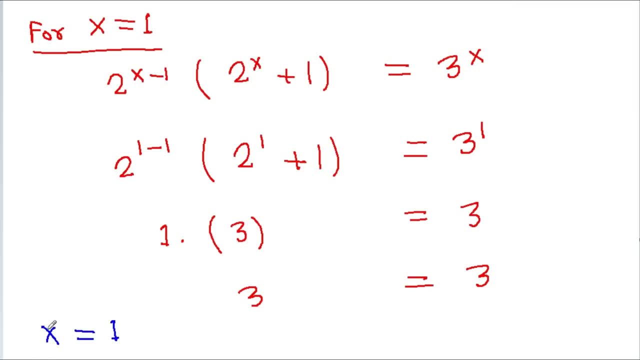 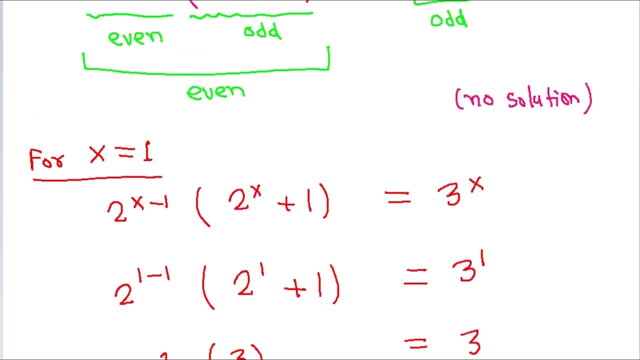 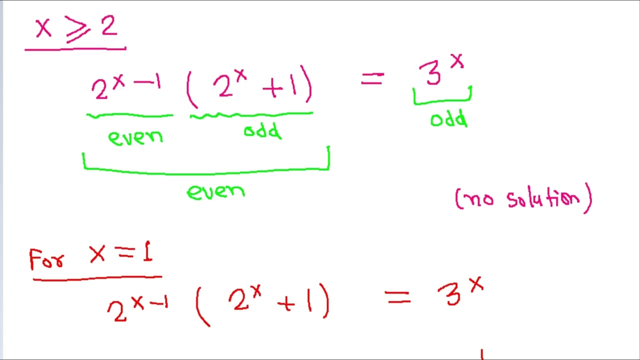 so x is equal to 1 is a solution. and now we have to check for negative x. so suppose x is equal to some negative n where n is greater than or equal to 1, and now we have 2 to the power x minus 1 times 2 to the power x minus 1 is equal to 3 to the power x. 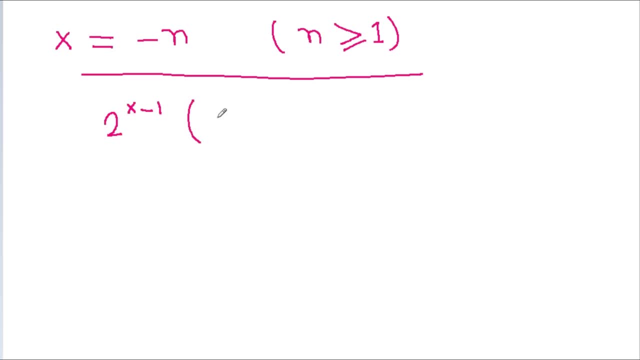 we have 2 to the power x minus 1 times 2 to the power x minus 1 is equal to 3 to the power x and for x is equal to minus n. it will be 2 to the power minus n minus 1 times 2 to the power minus n. 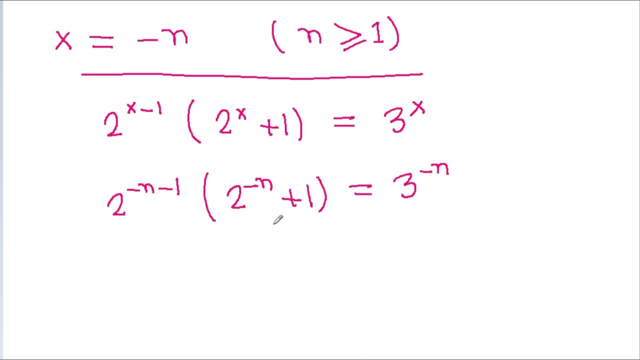 minus 1 is equal to 3 to the power minus n and 2 to the power minus n minus 1 will be 1 by 2 to the power n plus 1 into 2 to the power minus n is 1 by 2 to the power n. 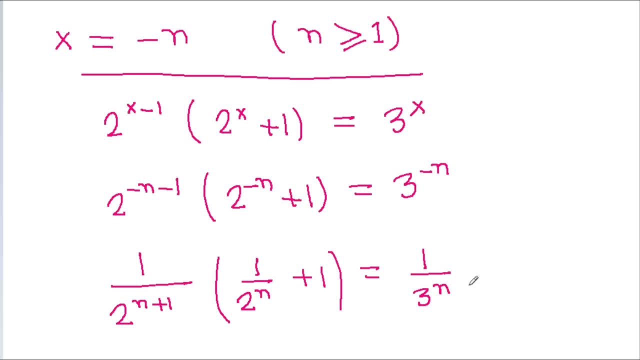 minus 1 is equal to 1 by 3 to the power n. and now we can get 1 by 2 to the power n minus 1 times 1 by 2 to the power n minus 1 times 1 by 2 to the power n minus 1 is equal to 1 by 2 to the power n. 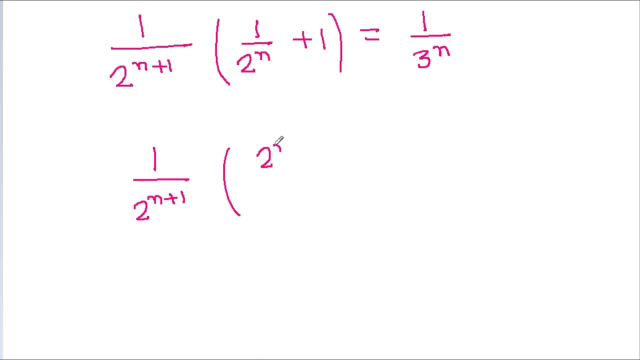 minus 1 it will be 2 to the power n minus 1 by 2 to the power n is equal to 1 by 3 to the power n, and now we can get 2 to the power n minus 1 by 2 to the power n minus 1. 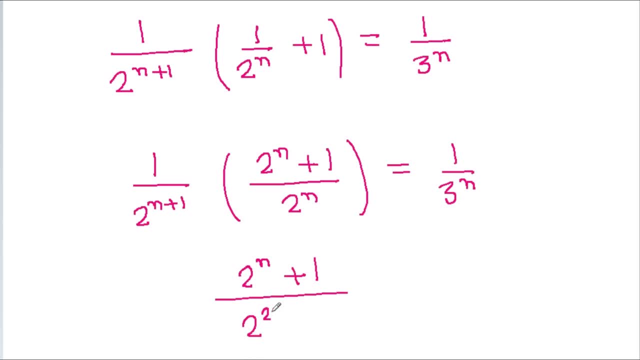 times 2 to the power n, it will be 2 to the power 2. n minus 1 is equal to 1 by 3 to the power n. and now if we cross multiply then we can get 3 to the power n times 2 to the power n.